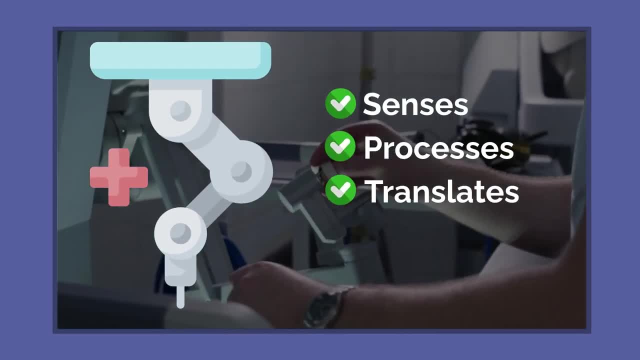 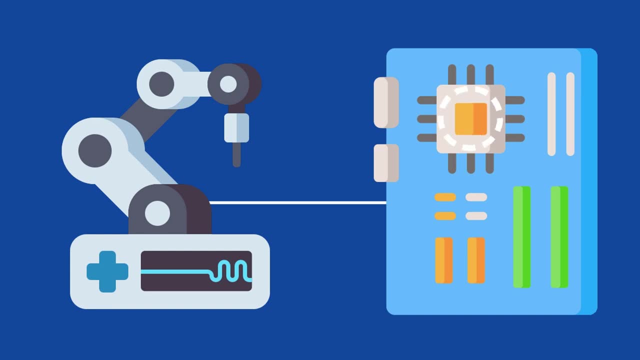 The entire system that senses, processes and translates the doctor's action to its own is all inside the surgical arm. In other words, the entire system is embedded in a system that is embedded right into the device. Now, if you think that's cool, then just wait until we deep. 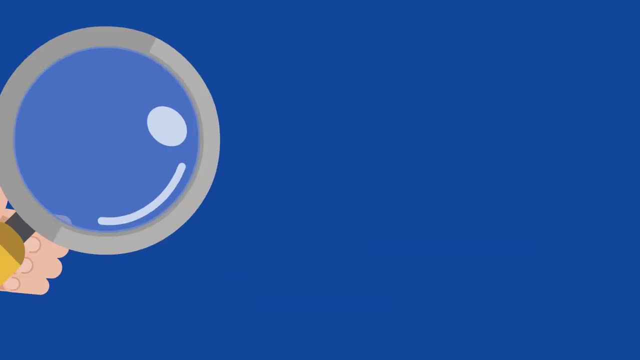 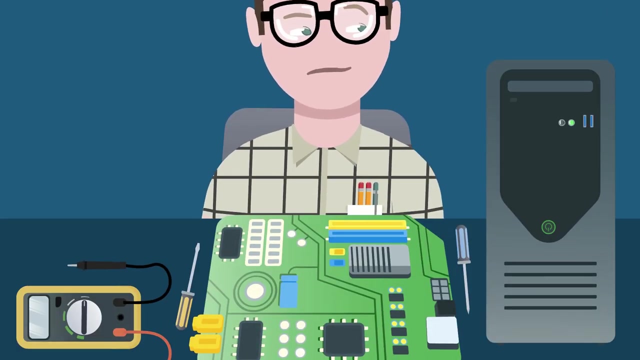 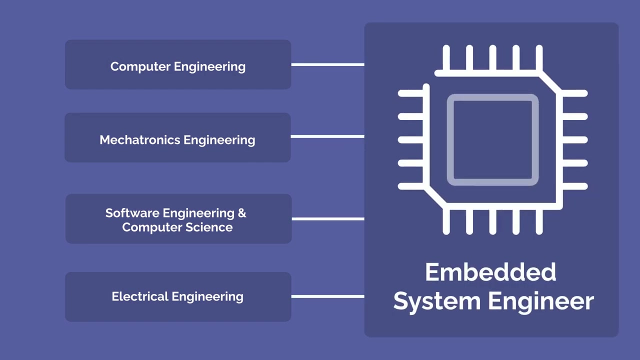 dive into the industry-leading GoPro action camera, highlighting what makes this embedded system such a remarkable feat of engineering. But before we get into that, we get to inspect how these engineers hone their crafts and reach wizardry status in the engineering world. Now there are a few university paths that typically lead to a career in embedded systems. 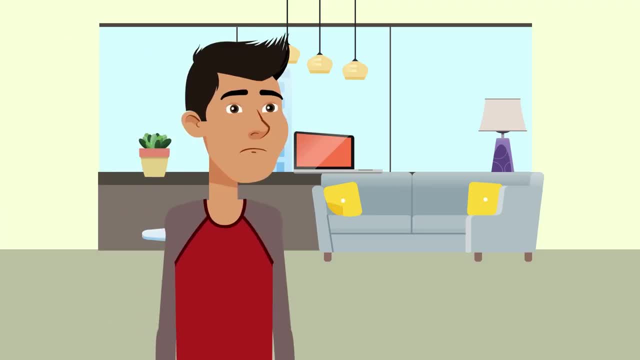 but the most relevant is definitely computer engineering. Make sure to not get discouraged if you're looking into embedded, and don't forget to subscribe to our channel for more videos like this. If you don't have the right degree, you can become an embedded engineer or any engineer for that. 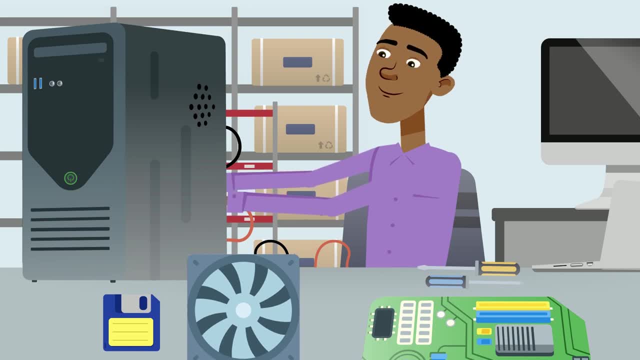 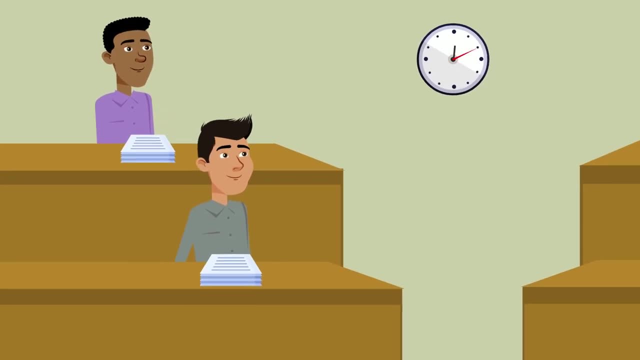 matter if you're willing to put in the extra work to train yourself, But what work do you have to do to become an embedded engineer? Great question. Let's discuss the most imperative college courses to take for aspiring embedded engineers. Now let's start it off with a fan. 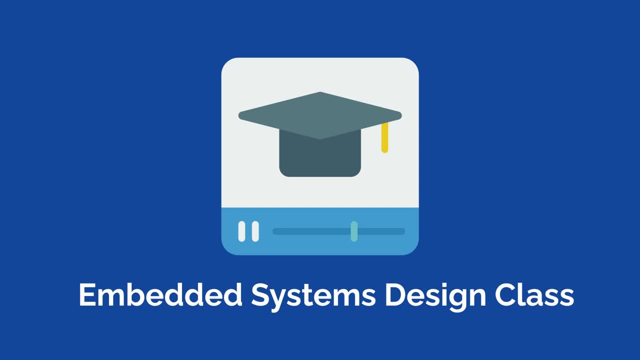 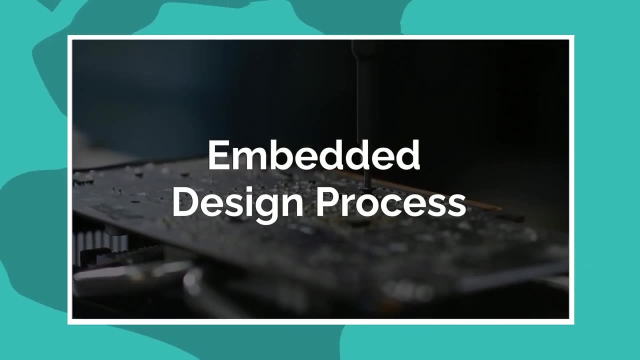 favorite, the Embedded Systems Design class. Just like it sounds, this course mimics a real-world embedded design. In the next part of the video we're covering everything to do with the embedded design process, So sit tight to hear the details for this one. But there's not going to be much sitting and waiting. 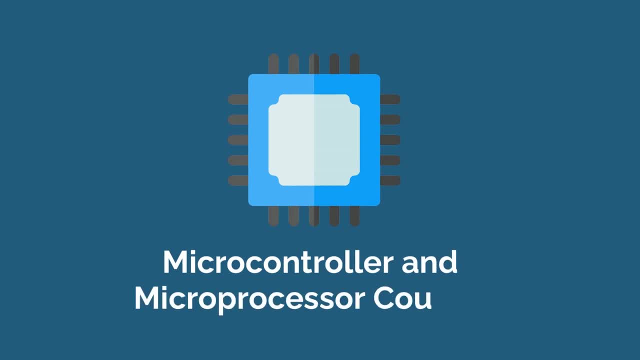 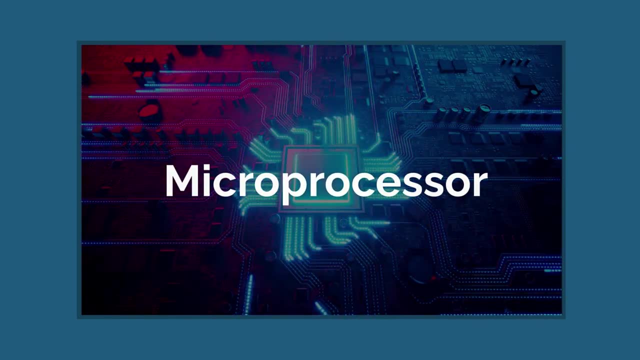 in your embedded degree You've got microcontroller and microprocessor courses up next, The heart of any embedded design is a microcontroller or a more simple microprocessor, which are typically programmed in the C programming language. Here you'll gain a ton of insight into controlling. 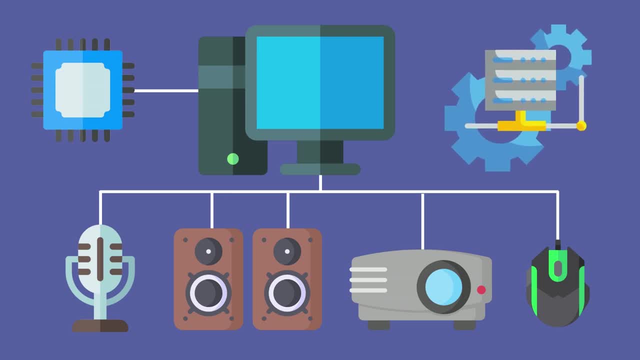 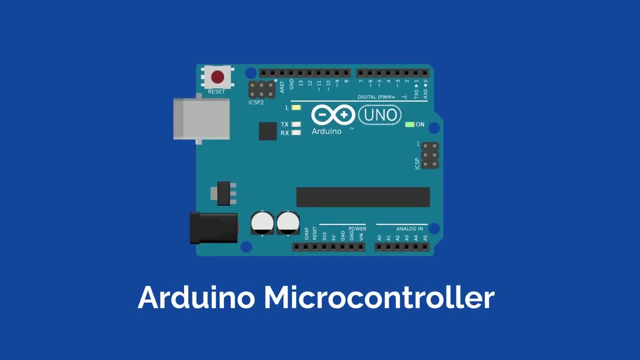 peripherals with a microcontroller and the C skills necessary to get it done. If you want to practice this extremely important skill from home, we recommend trying out the beginner-friendly Arduino microcontroller- From simple LED circuits to developing robots and homemade 3D printers. 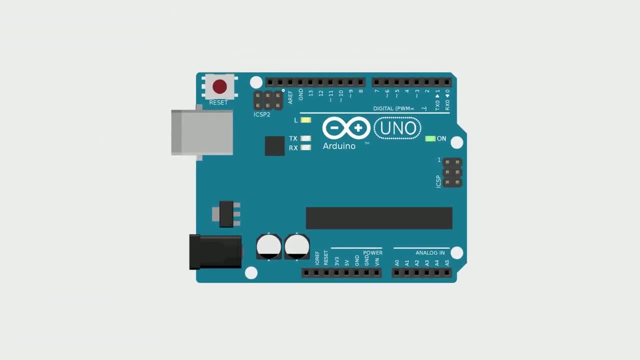 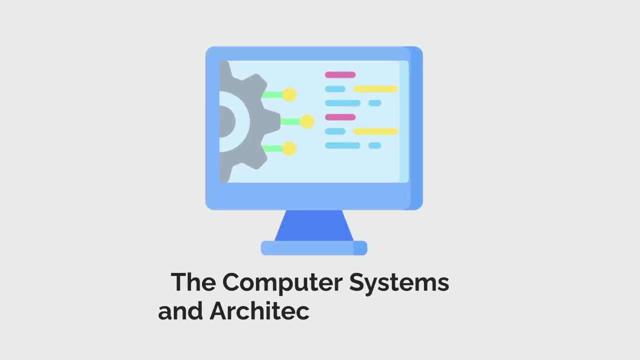 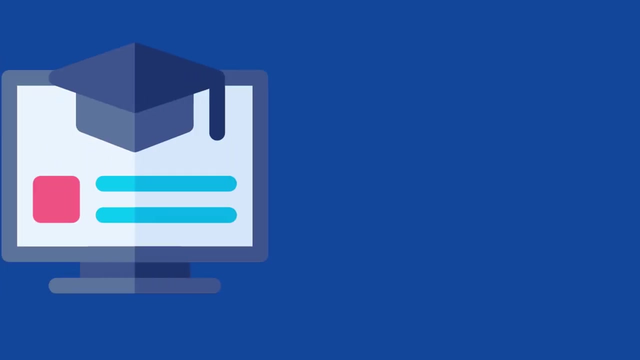 Arduinos give a great indication of any microcontroller-related field for all skill levels. Check out the resources in the description if you're interested. Next, the computer systems and architecture courses are a must-have, giving a detailed perspective on all the electronics that go into making a computer. Further, these courses: 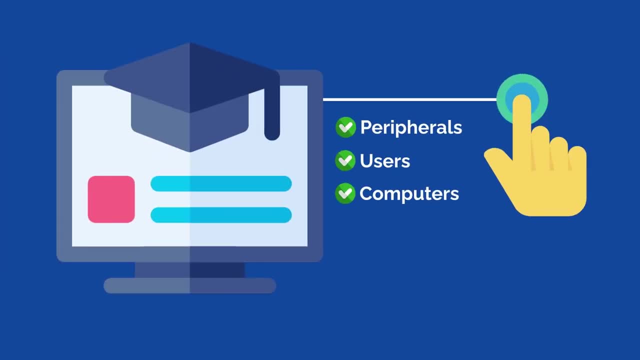 teach you how to interface with peripherals, users and even other computers. Similarly, it is imperative that you take a look at the interface between the computer and the computer. It's important that you take a low-level programming class so you understand enough machine language. 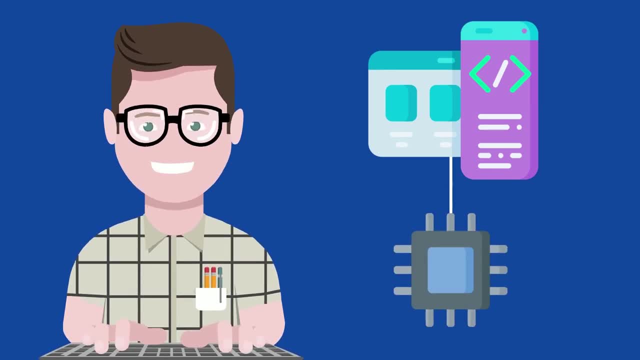 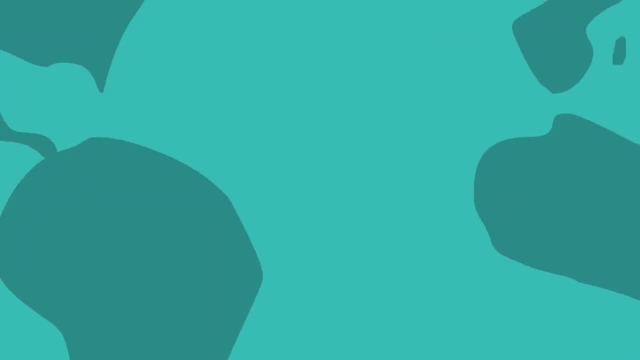 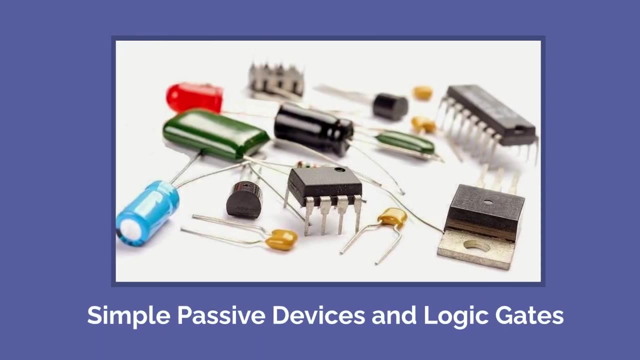 to control the hardware in your embedded designs later on. Most embedded engineers need to know a healthy chunk of circuitry as well for hardware design and debugging, which leads us to the shocking world of analog and digital circuits. Topics in these courses include everything from simple passive devices and logic gates to more intricate circuit schemes. 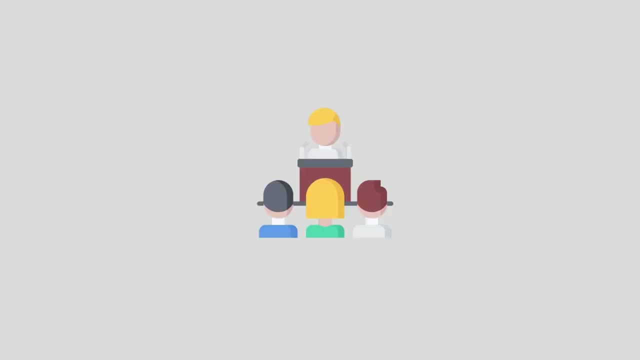 that really get those oscillators teetering. The last classes we'll touch on are extremely important to embedded engineers: Data structures and algorithms. Debatably, the harshest constraints of embedded designs are the time and computing power that your programs consume Without a structured 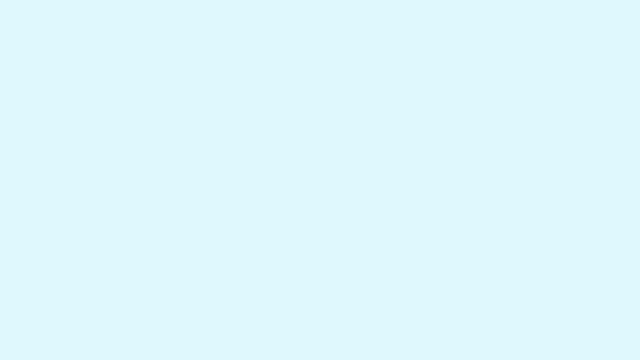 background for efficient practices and structures. you'll be treading water trying to figure out how to squeeze a 50-microsecond program into a fraction of that time. Now, of course, there are other important math, physics and engineering courses that 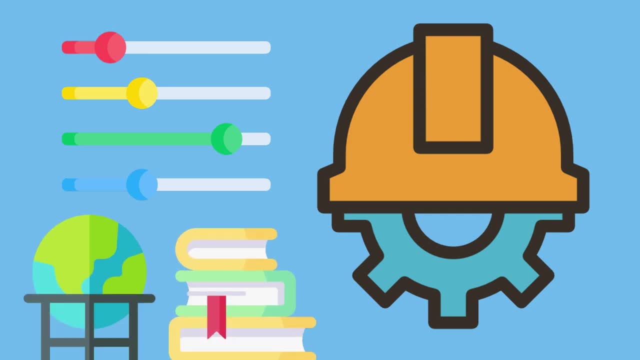 have varying levels of real-world help for your career, But the ones we just covered are pretty much the must-haves. Next, the computer systems and architecture courses are a must-have, giving a detailed overview of the world of embedded engineering. For more information, you can check out our. 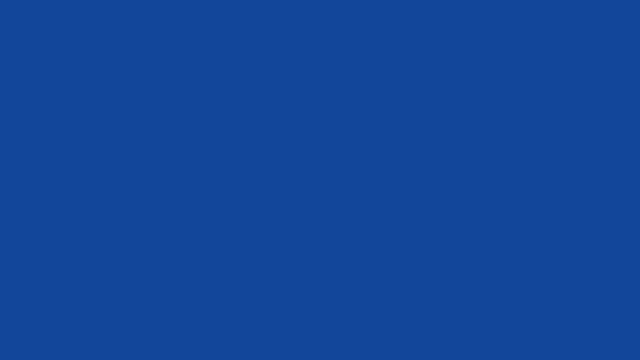 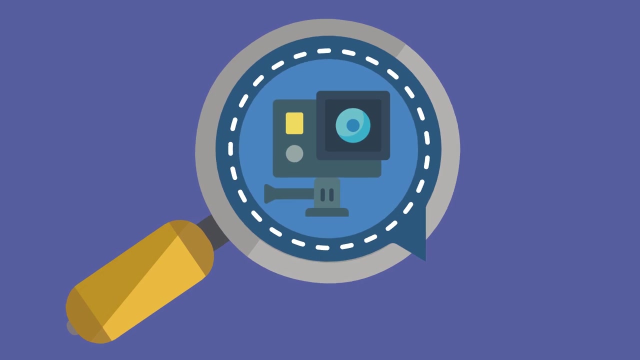 electrical or computer engineering curriculum roadmaps. But enough with the university stuff, Let's get our hands dirty with that real-life embedded engineering design. Just as promised, we'll be investigating the fascinating details of a GoPro digital camera to carry us through the nuances of an embedded engineering design. We've simplified the 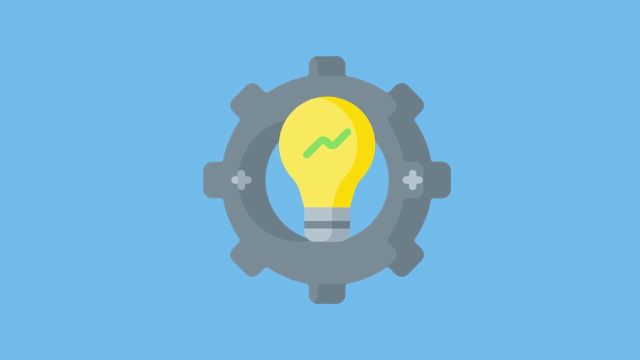 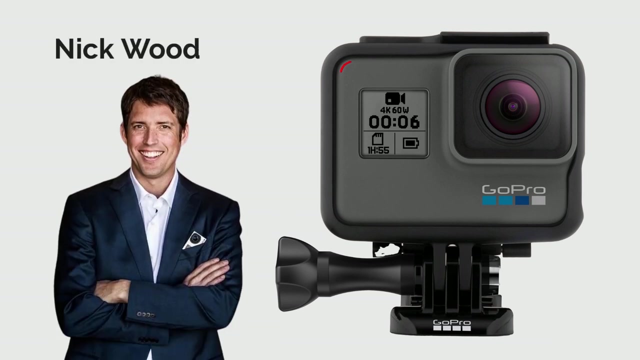 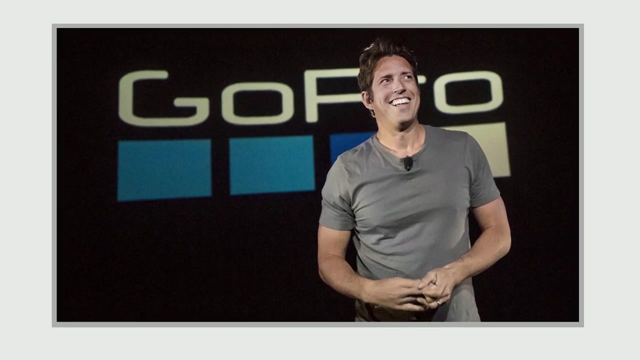 details. just a touch for the sake of the video, but all the core concepts hold true. Without further ado, let's get right into it. It all started with GoPro founder and California native, Nick Woodman, hatching a brilliant idea that would eventually cement the dominance of embedded systems in the 21st century. He 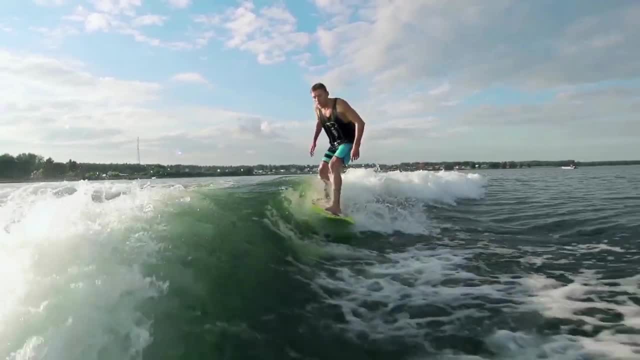 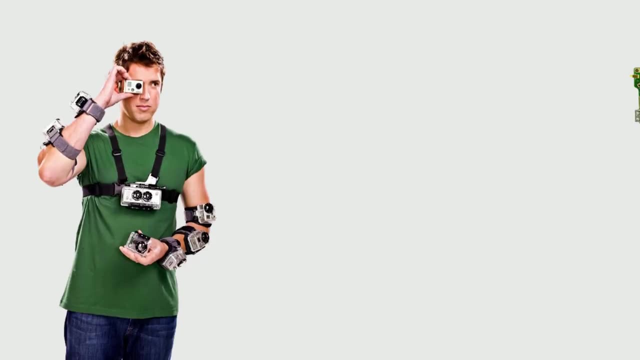 was simply looking for a better way to film him and his friend surfing, speculating that there would be a ton of others like them. with the need for a small but powerful digital camera, This idea perfectly set the stage for a world-class, multi-million-dollar embedded system design. 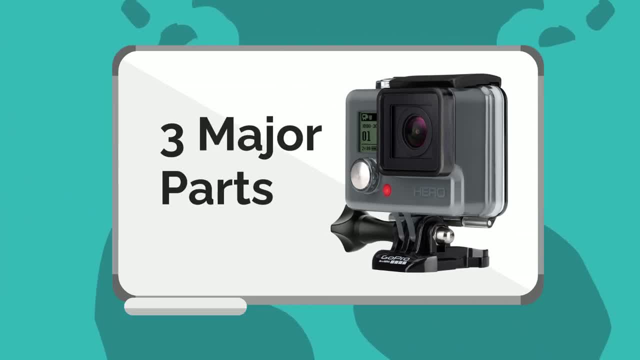 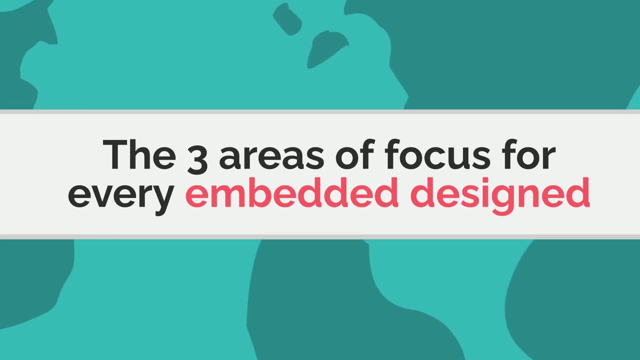 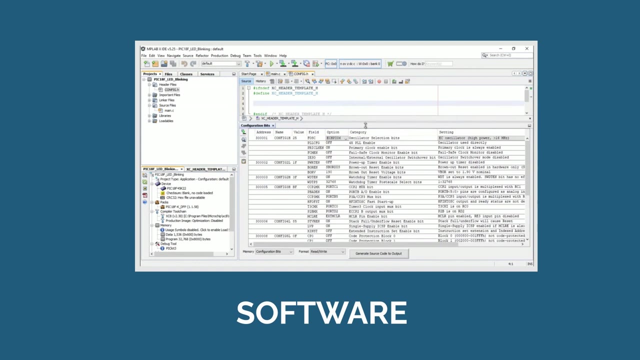 They went to the drawing board and decided upon three major parts of the camera to start designing, which are consequently the three areas of focus for every embedded design. So make sure you're paying attention here. They are the hardware that can film and store quality videos, the software that controls the process and interfaces with users, and 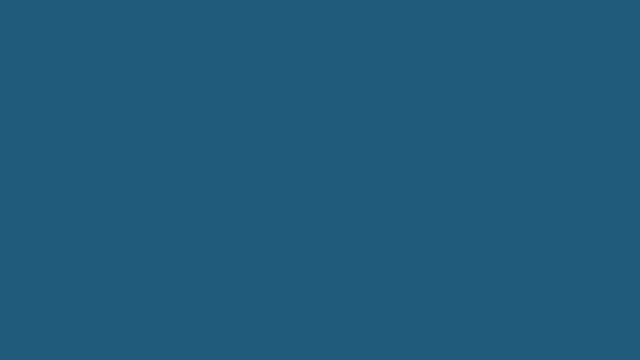 the compact, rugged casing to protect the technology inside. But what is the technology inside? What are the embedded engineers actually designing? Okay, let's explore that, Starting with the most obvious part of the camera. we got the lens. The engineers took 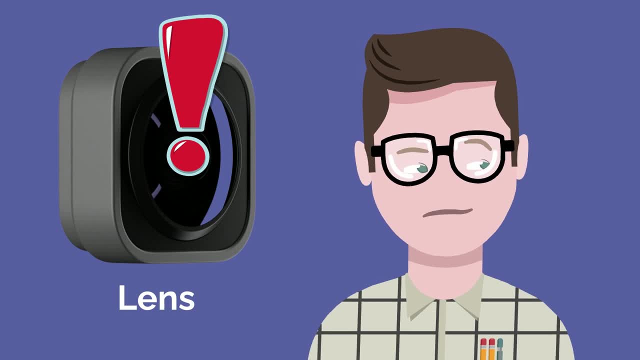 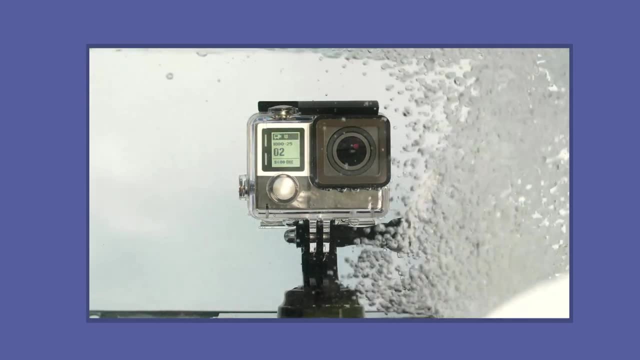 their time choosing this part, as it's the single most important input for the camera: The light reflected off the subject to be stored as a video. Once this light is herded into the body of the camera, it needs to be transformed into an electrical signal, so our embedded 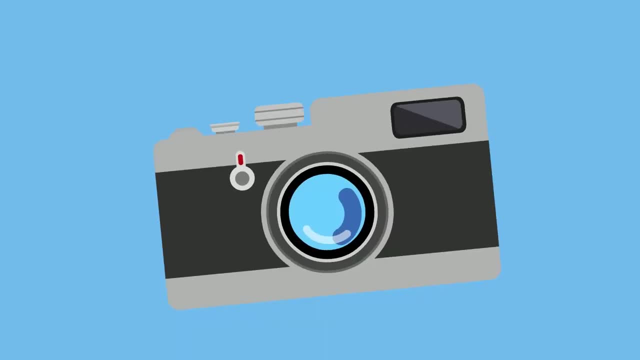 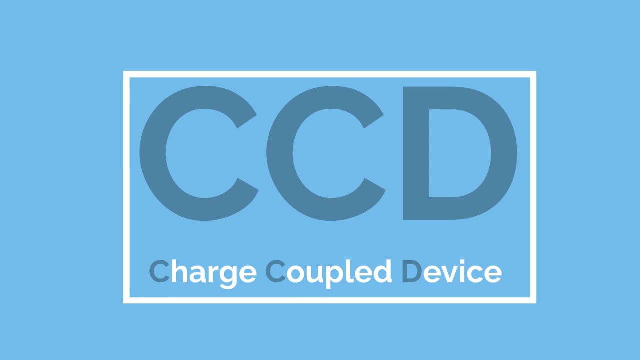 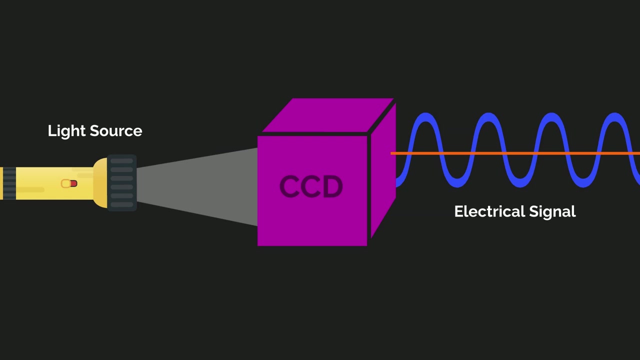 technologies can manipulate and store it. This transformation from light to an electrical signal is accomplished with a CCD or charge-coupled device. Basically, this CCD has an entire field of discrete points that light hits, and each point emits a current proportional light. The embedded engineers chose the single best CCD for the design, as there is simply. 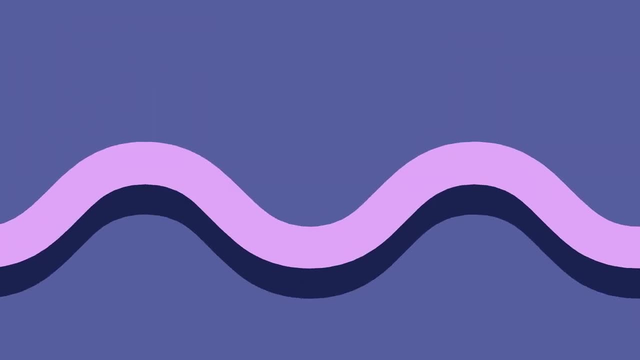 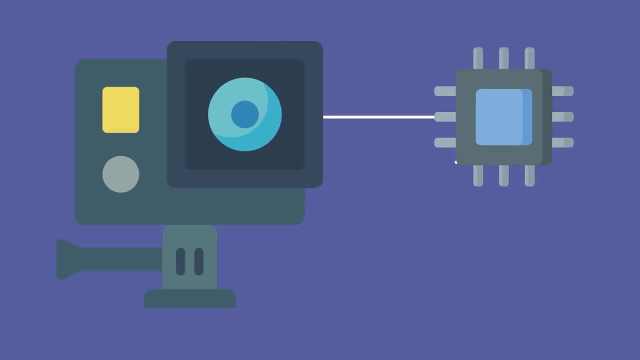 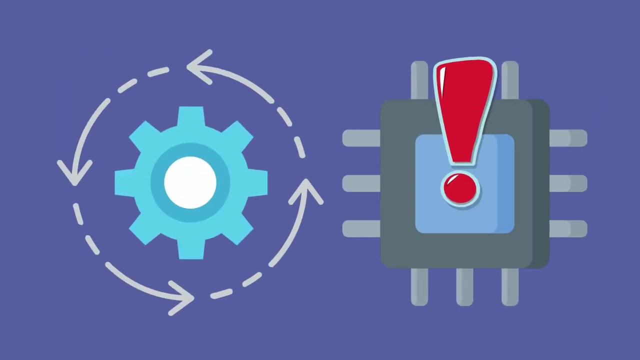 no room for inefficiencies in this small camera. The electrical signal from the CCD is routed through an analog-to-digital converter so that the GoPro's brain, the processor, can interpret the exact levels of light that the lens initially captured. Like previously mentioned, the processor is the most important part of 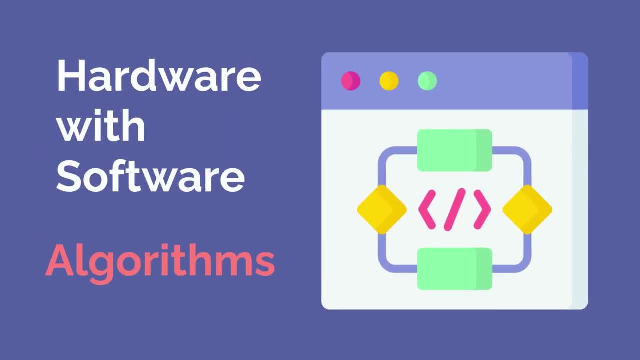 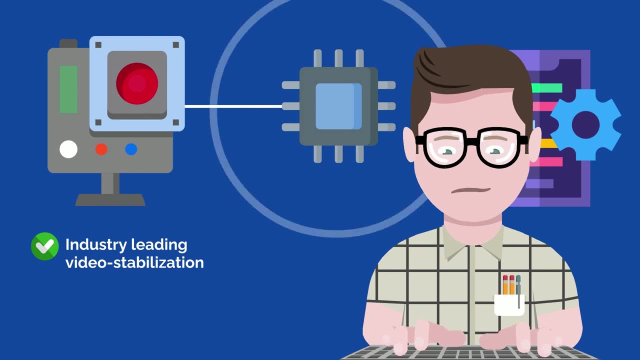 the system as it ties together all of the hardware with software algorithms. The embedded engineers chose and programmed a processor that can accomplish their industry-leading video stabilization, logging the high-quality video to the camera's memory and many more tasks never seen by the user. 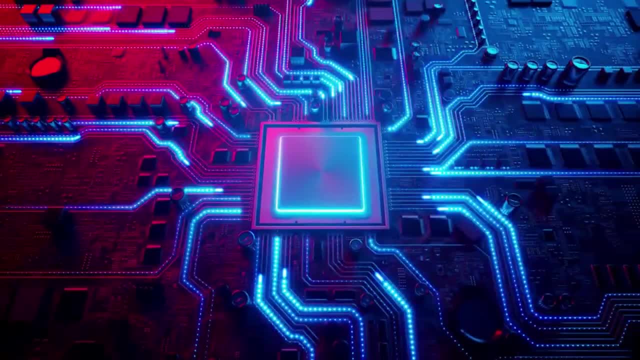 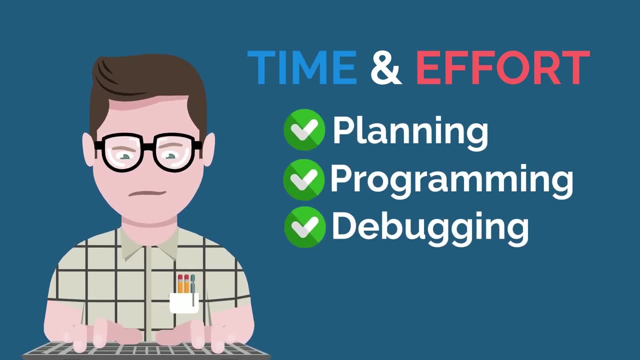 Seeing as the processor is the integral core of the entire system and is extremely challenging to aptly control. most of the embedded engineers' time and effort goes into the planning, programming and debugging right here in the processor, which leads us right into the perfected software. 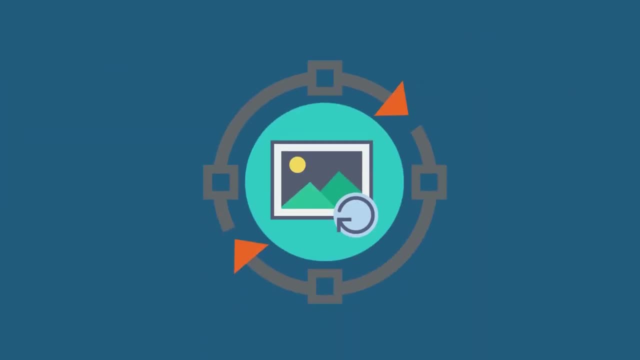 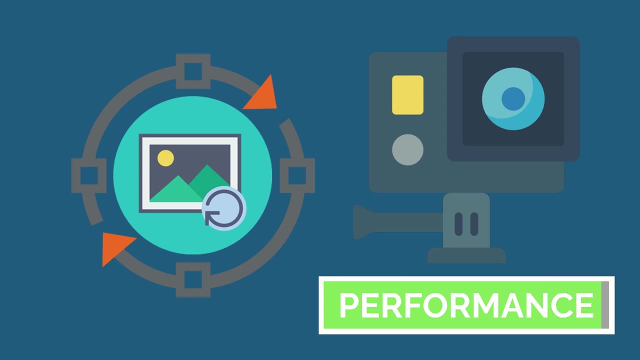 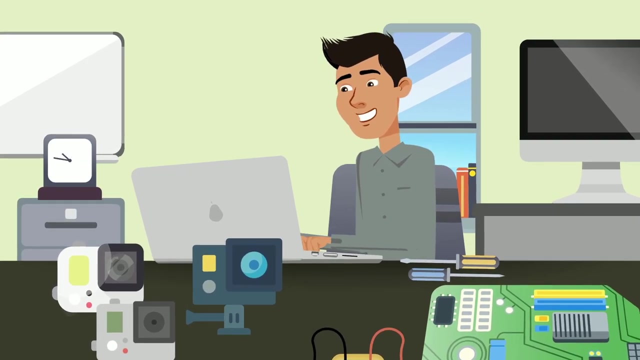 of the system, From configuring the start button to the vast image processing algorithms, each and every algorithm has been decidedly chosen to optimize the camera for maximum performance, cutting out any operations that aren't absolutely necessary to the success of the device, Without an immaculate attention to detail. among these tens of thousands,